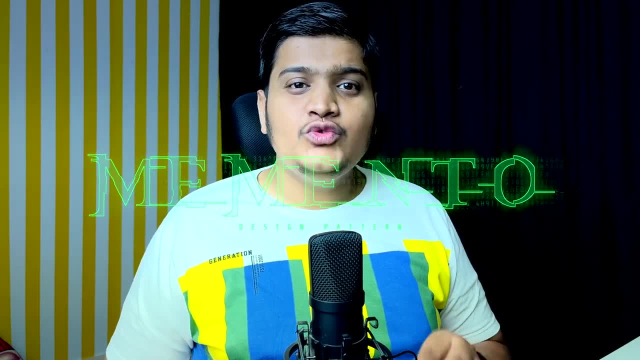 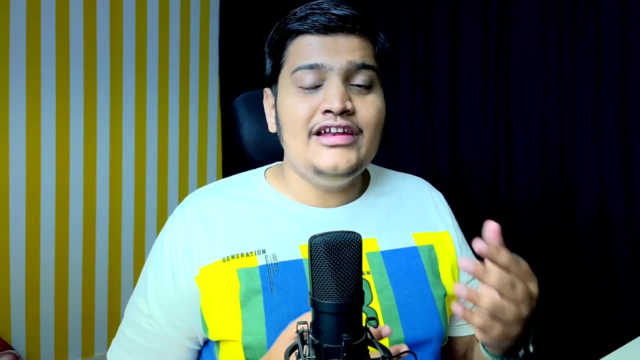 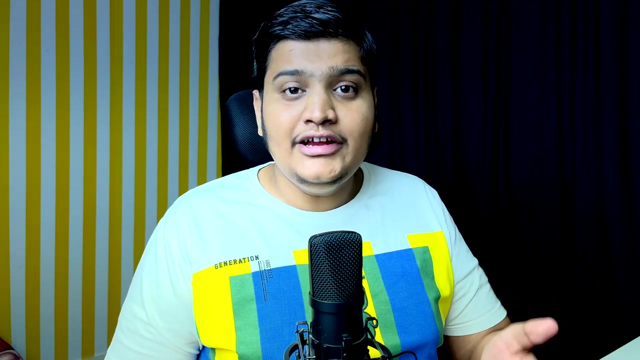 Hey, what's up everyone and welcome to daily code buffer. In this video we are going to see about the memento design pattern. So memento design pattern is a part of a behavioral design pattern and it is used when you have to store the state of your objects and you have to have the capability. 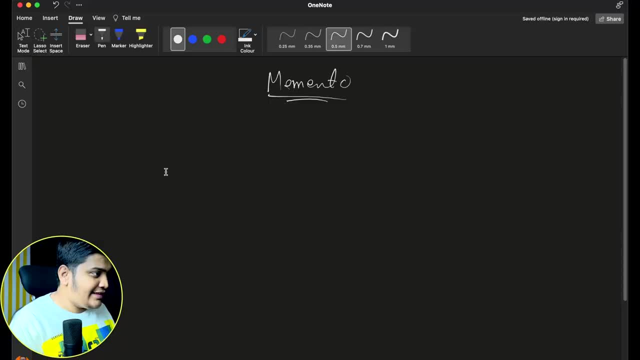 to restore those objects as well to the previous state. So, taking the example that you have the different objects available and you are storing the states of the particular objects, So suppose you are storing state 1, state 2, state 3.. These are the different states that you are doing on. 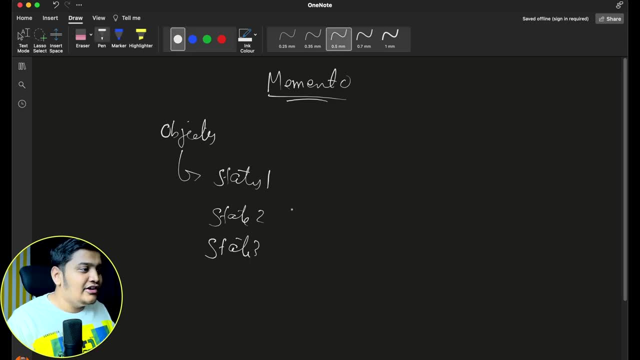 your object- So there are different modifications on your objects- and for your application to have the capability to restore this particular previous state- Suppose you want to restore to state 1, you want to restore to state 2 and so on. Okay, if you want to have those capabilities, at that time we 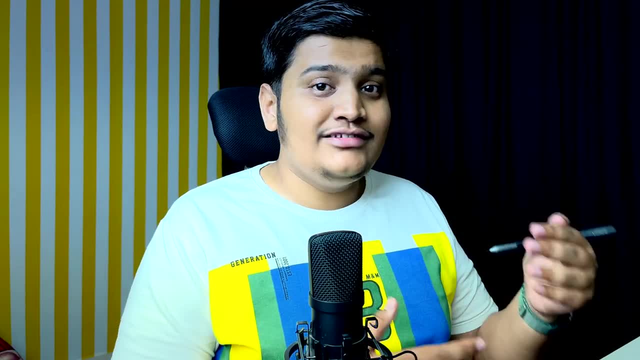 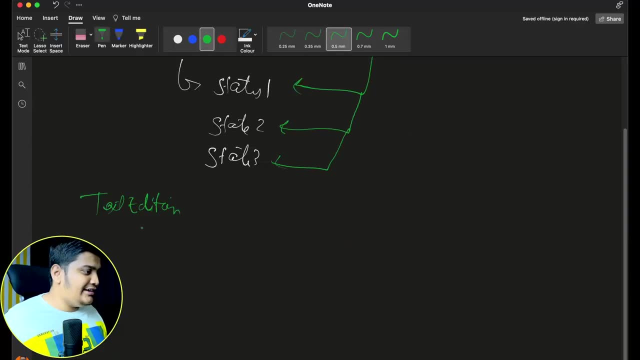 will implement the memento design pattern Now, when you will need this. what is the real-time example? So real-time example is like: take the example of a text editor. You have the text editor and for that particular text editor, you have the object right, All the things happening within your text editor. 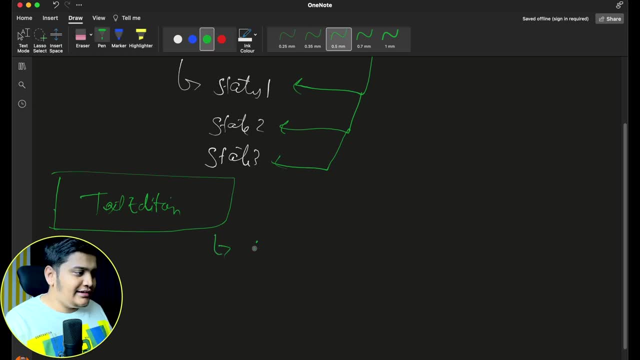 will be stored here. Okay, so suppose you are storing what is the text here like, what is the data that you have been stored and what are the number of lines and all those information. you will store the line number, at which particular line you are at, or you will also add the scroll. 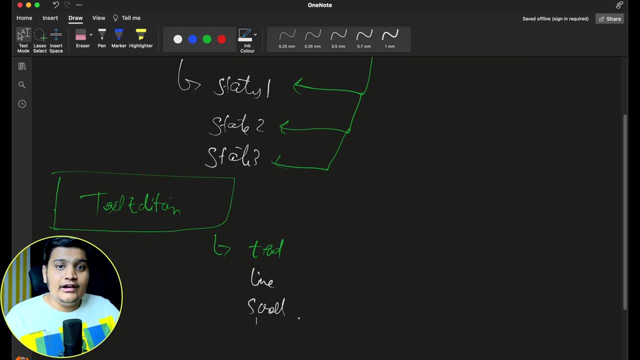 positions like what you have scrolled within the page. If you have written a lot of data, then there will be a lot of data stored within the page. So if you have written a lot of data, then there will be a scroll as well, right? So all those information you will store, and whenever you are doing any, 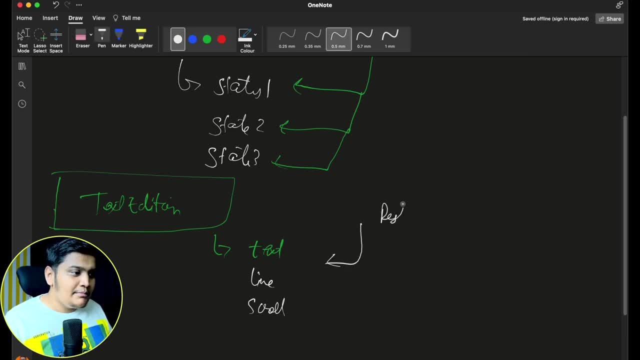 mistake. what you have to do is you have to restore to the previous positions as well. Okay, so if you want to restore what was there earlier, you have to restore to the previous position as well. Now, what will happen with this is there are two types of senior scenarios, like either: for all the things, 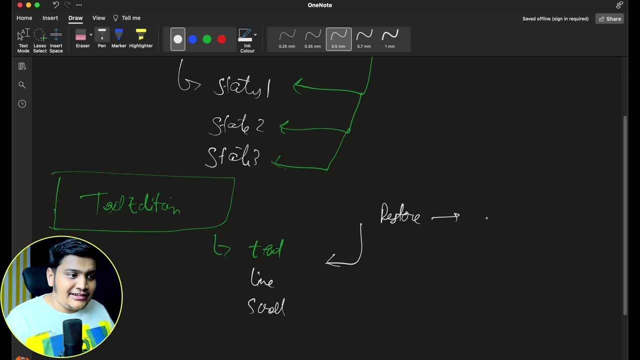 that you have defined here within the text editor. either you give the access of each and every fields- Okay, access to each and every fields to identify what is the text editor and what is the change and what needs to be changed, or you give all those capabilities to a different class and 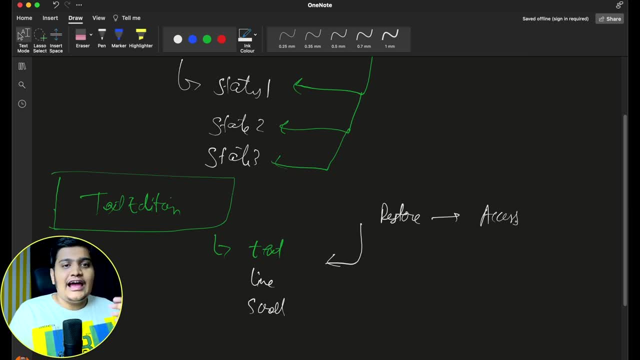 that particular class will identify what are the changes and it will help us to restore to the previous state. Okay, so these are the different ways: giving all the access, all the fields, making as a public. it's not a good idea, right? So that's why we are using the memento design pattern Now. 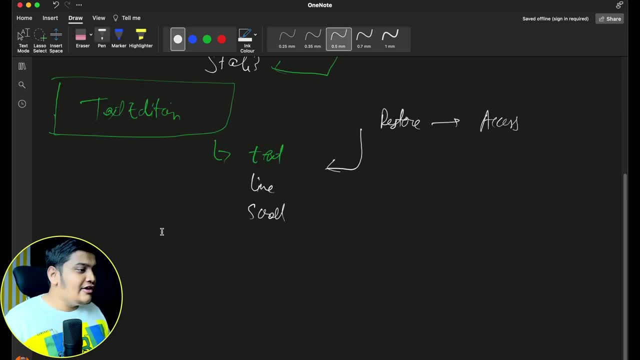 what generally we will identify within the memento design pattern is for any state that you want to store. There are three different classes that we are going to use, So we are going to use the create here to implement the memento design pattern. One would be the memento: Okay, memento. 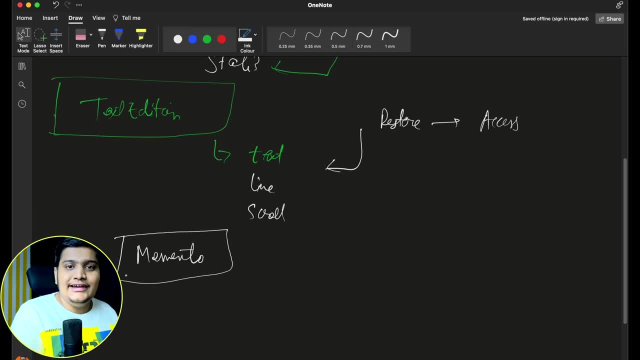 means the state itself. Okay, like what particular state it is? I want to store a state of that particular object. that is my memento. I will store that. Okay, one will be the originator, like: who is creating that particular state? Okay, who is creating that particular state and this particular? 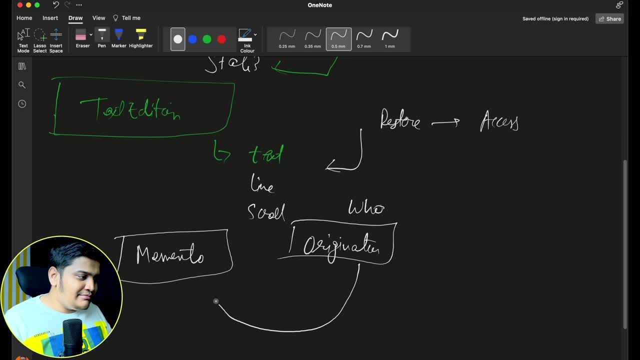 part, will be responsible to store that state in my memento as well, Like: what was the state of that particular object? Okay, and one would be the caretaker. This caretaker will be responsible to restore my state, Okay, so whatever the states are there for within, 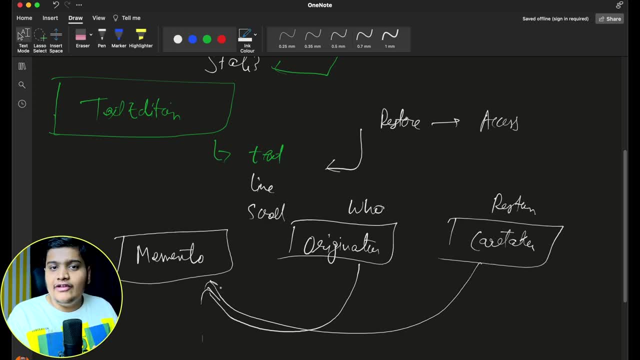 the memento. if anything I want to restore, caretaker will be responsible for me to restore to that particular previous state. Okay, whatever I want to do. So this is what we are going to create, what is memento, originator and caretaker, and these are the different classes that we are going to. 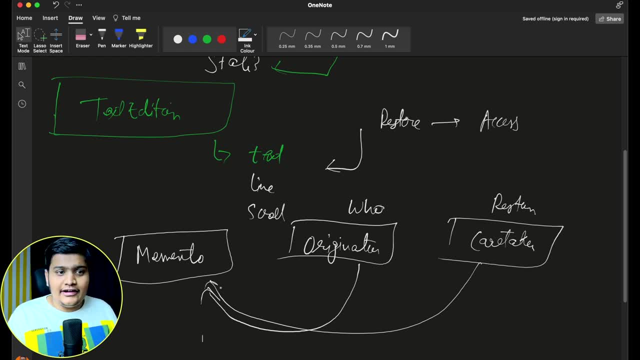 create and there will be a client class which is going to call originator and caretaker, and memento will not be directly used because that will be your state machine right. all the states will be defined there itself. Okay, so let's check the example. we'll go to the IntelliJ IDEA and let's see that. 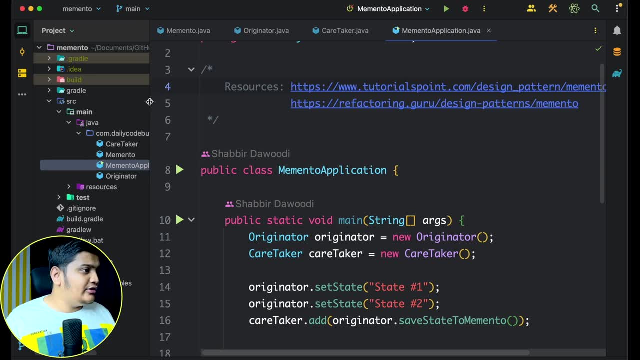 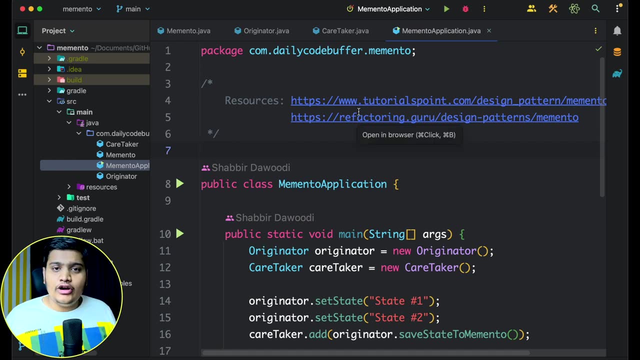 example. Okay, so here you can see that I have opened the memento design pattern here and I have taken the references from the tutorials point and refactoring guru. I've added the resources as well, so if you want to check them out, you can check them out as well. Okay, I will add all the links. 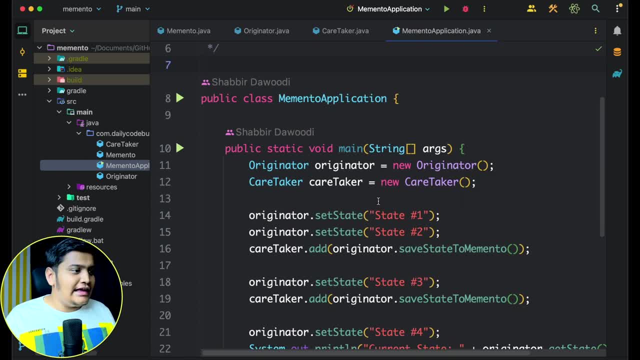 in the description below for you to check out. Okay, so let's go ahead and let's go ahead and check out. I will add the link for this code as well, and this is the entire code I have taken from the tutorials point. So here you can see that I am creating a memento here. Okay, this is the first. 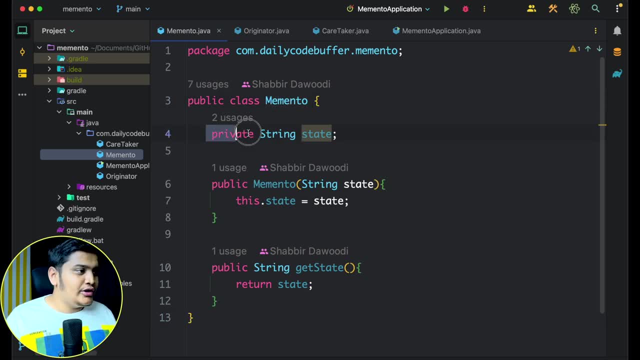 thing that I am creating and within the memento, you can see that I am storing the state, What is the state? and for this state, you can see that I have the memento constructor, which is taking the state and assigning the state here, and I have the method to get my state. Okay, that's a simple thing. 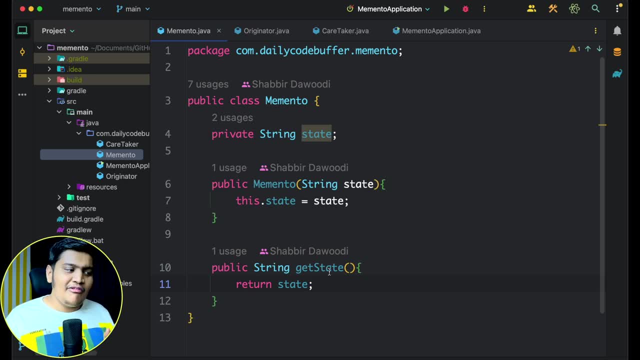 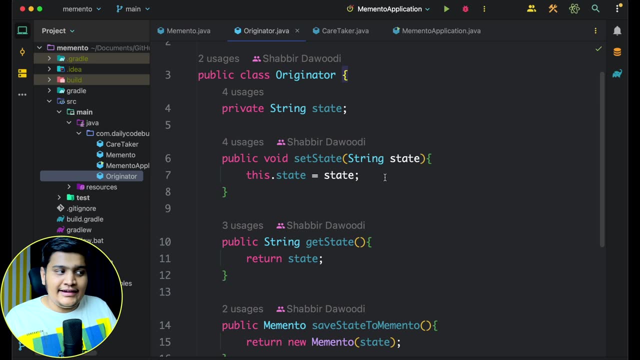 there is no setter. everything I will set within the constructor and I have a method to get my state okay. now let's see about the originator. Originator is responsible to save my states. okay, so this is the class originator and this originator have the reference of the state. what state I want to store? 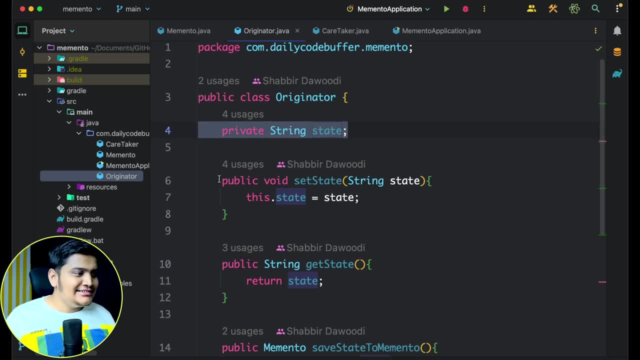 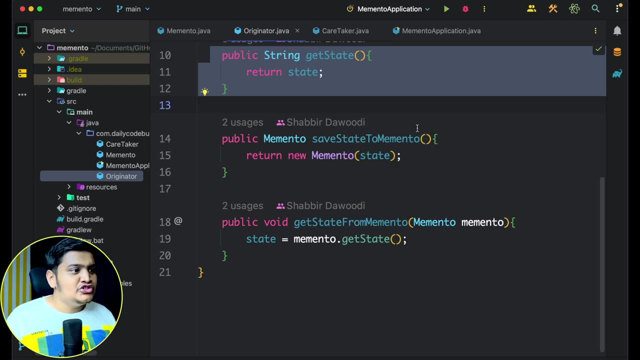 so you can see that within for this state, I have the set state method and get state method as well. okay, two methods I have, and I have a method save state to memento as well. so whenever there is a state change, okay, you can see that what I will do is I will save state to memento. I will call this. 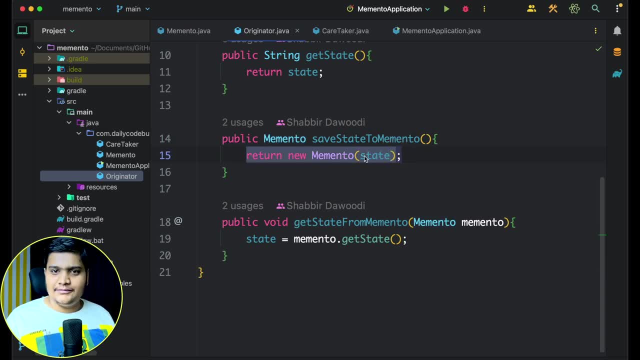 return a memento and it will pass the state here. okay, that's a simple method that it will save state to memento, will return a memento and it will return the object. and there is a method: get state from memento. so, whatever the memento that you will pass here, it will return the state from that, okay. 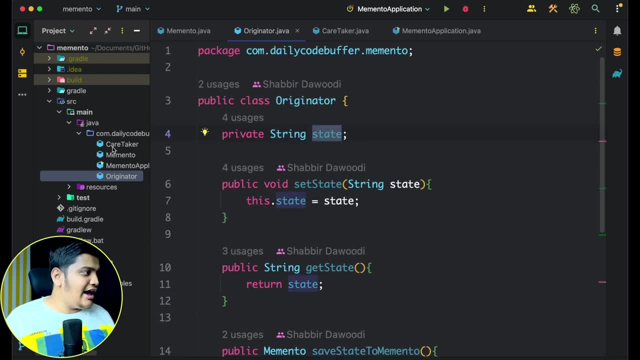 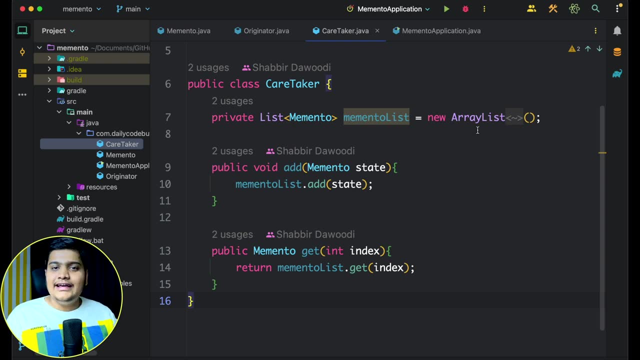 and it will store the state here within this originator and we have the caretaker method. you can see that caretaker will have all the memento here and it is responsible for you to get that memento, to restore it, okay, so this caretaker has a list of memento here, okay, and it has a method add. 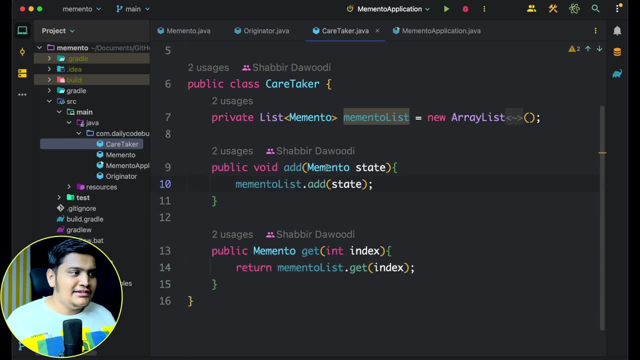 memento and get memento. okay, so you will just pass the memento here and that memento will be added in that particular list and if you will pass the index like which particular state you want, that particular state will be returned from here. okay, these are the three simple classes that we have. 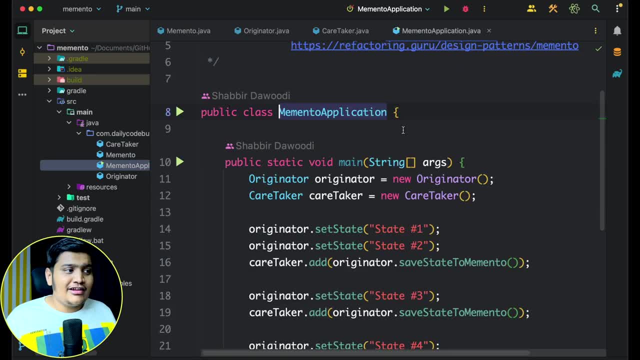 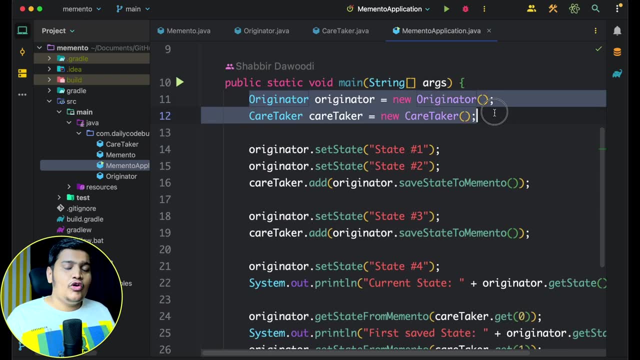 created. okay, and let's see how we can use it. okay, so this is our client application, how client will be able to call it. okay, so you can see that we will be just calling originator and caretaker. we won't be directly using memento class. okay, so we just define originator and caretaker and with the